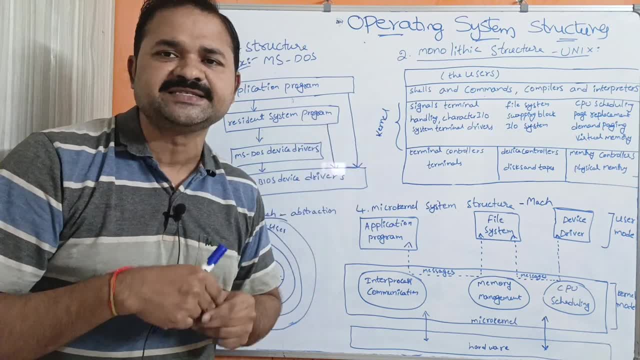 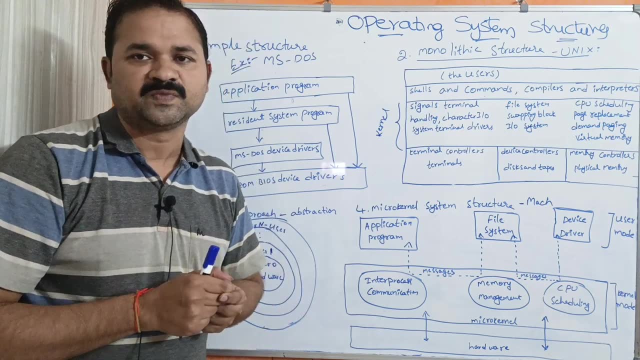 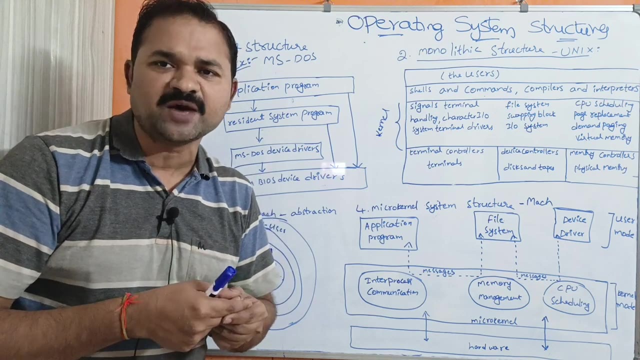 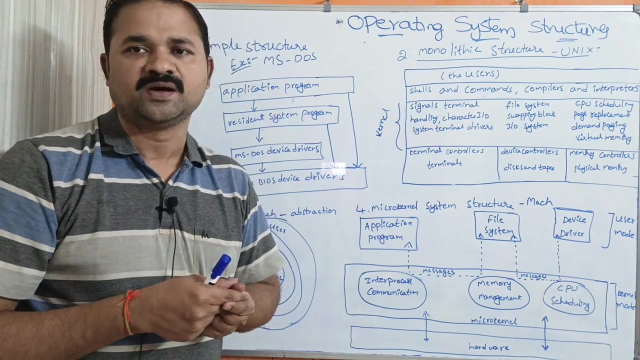 major advantage of MS Das operating system is in less space we can implement the functionality. But we know that the major disadvantage of MS Das is it is a single programming system. So that means at a time CPU can execute only one program. After executing that program, only CPU can start executing. 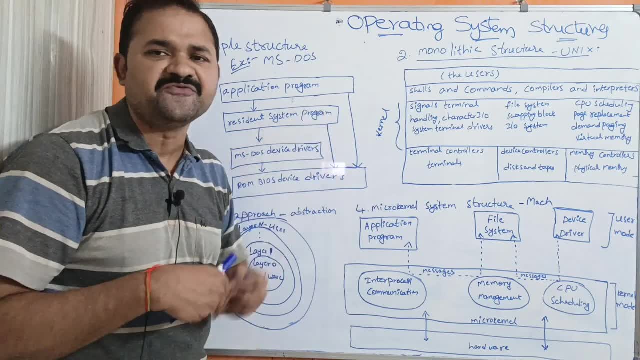 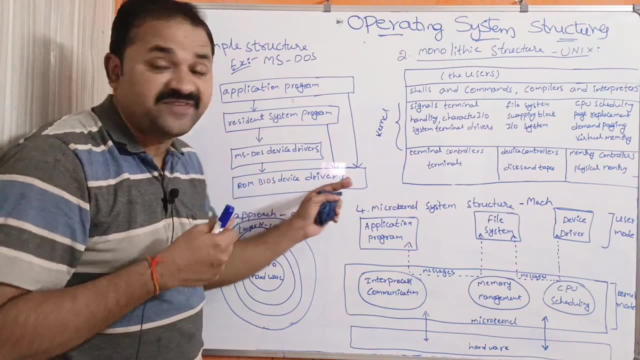 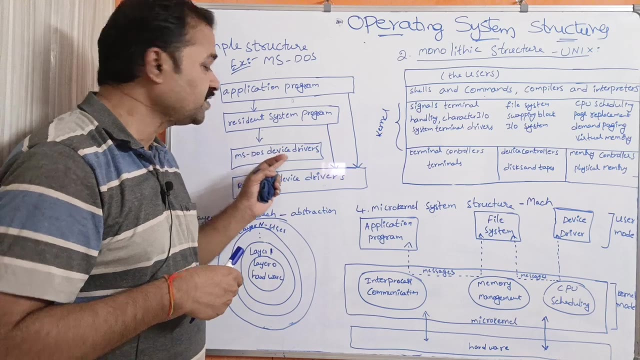 some other program. Now let us see the diagram for the the MS Das. Here the bottom one is ROM BIAS DEVICE DRIVERS. So here the bottom layer is ROM DEVICE DRIVERS. On top of this we have MS Das DEVICE DRIVERS. On top of this we have ROM BIAS DEVICE DRIVERS. On top of 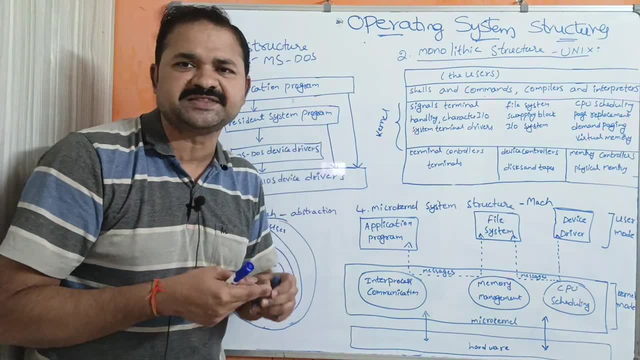 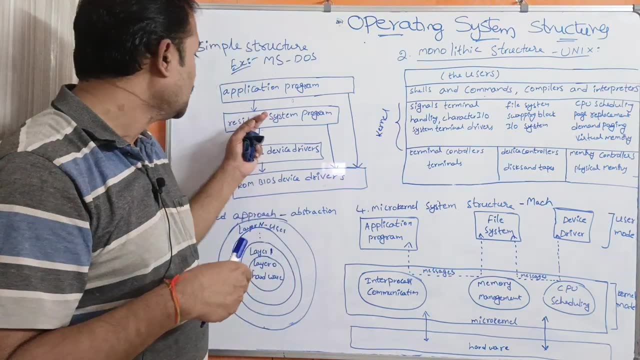 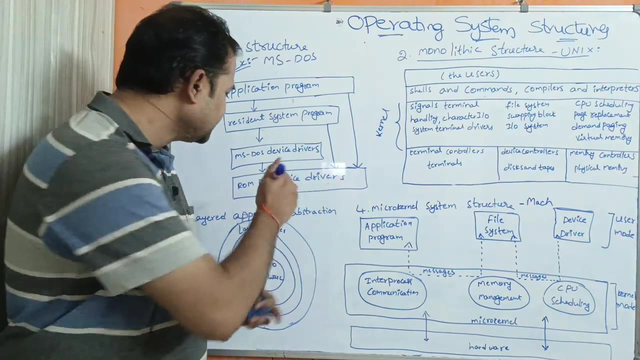 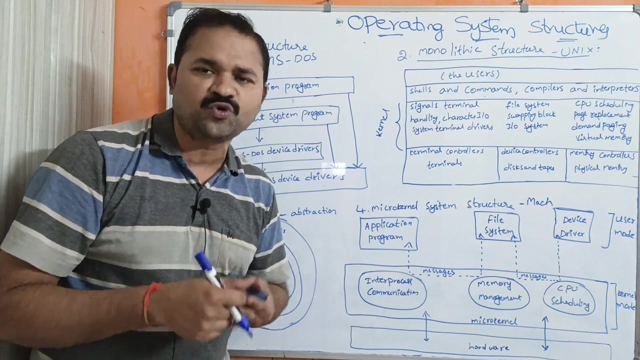 this we have resident system program. that is nothing but system program. the the most commonly system program is operating system. on top of this we have application program. here. application program can access this wrong device. drivers is nothing but hardware. we know that any computer mainly contains four components. the bottom layer is hardware. on top of it we have some operating. 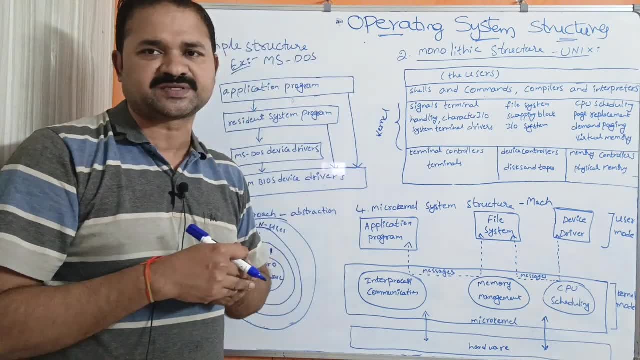 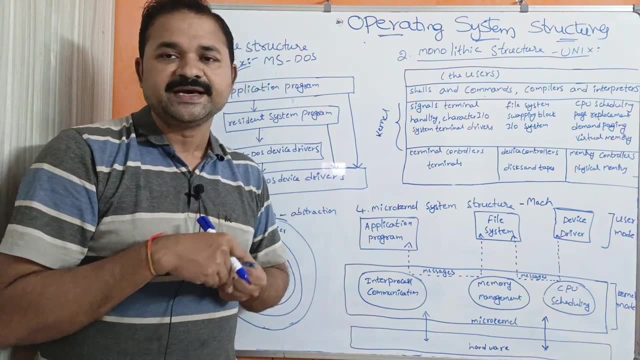 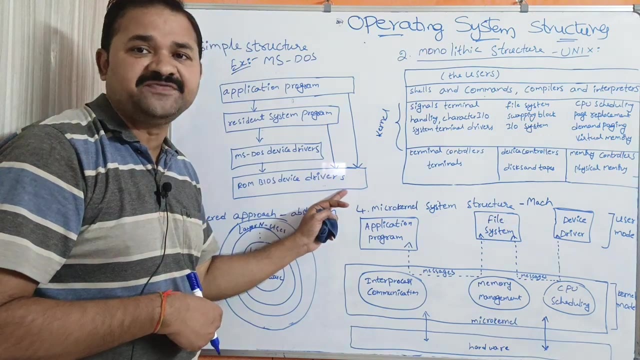 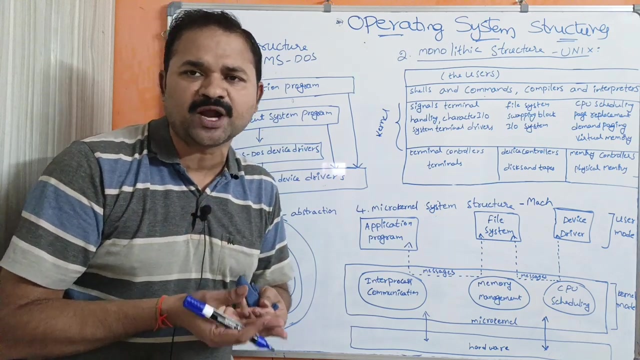 system. on top of it we have some application programs. so here this wrong bias device drivers is nothing but hardware components. here the major problem is an application program can access the hardware devices directly. so there is a possibility that application program may change the content of the hardware. so 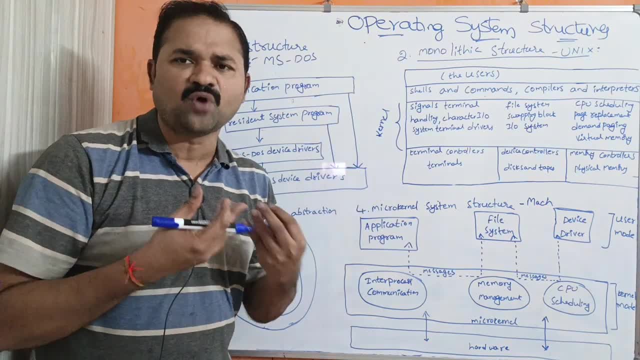 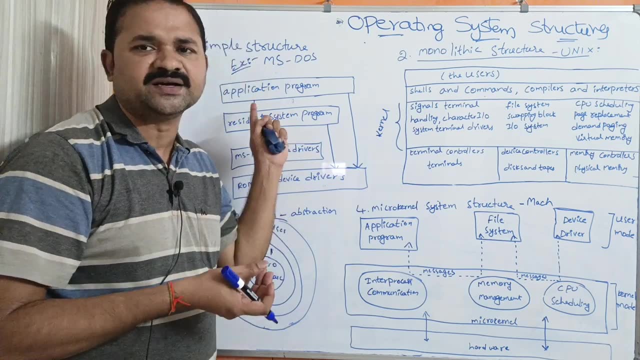 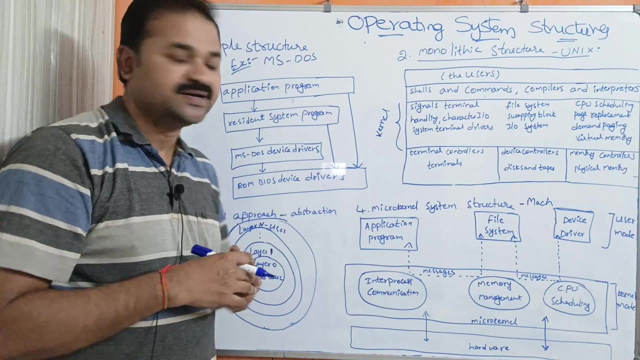 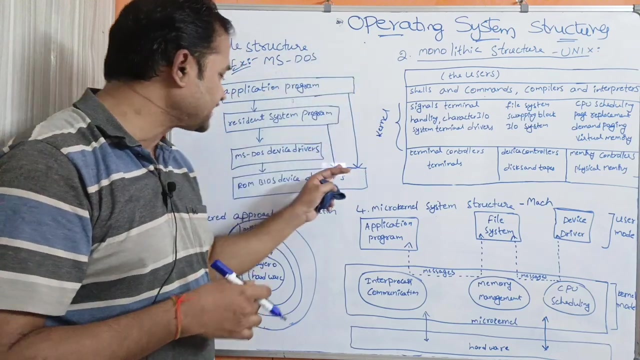 if, if application program fails, we know what is application program. application program is nothing but a program which is developed by the user. so we can say that if an application program crashes, fails, then the entire system will fail. why? because here the application program is has direct access with hardware devices. so this is the problem here. if our program 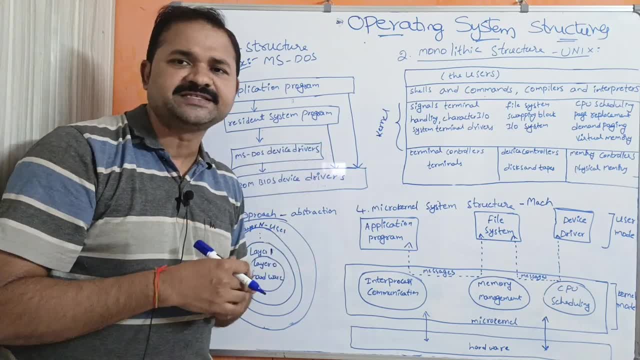 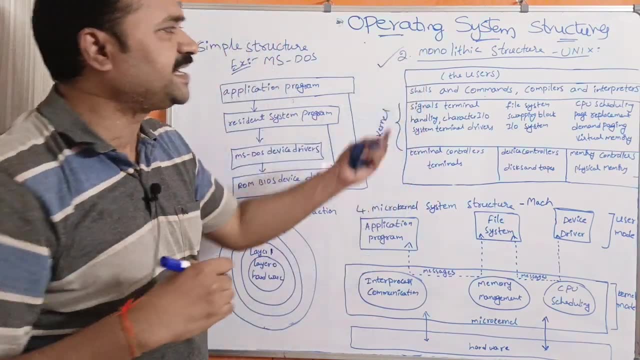 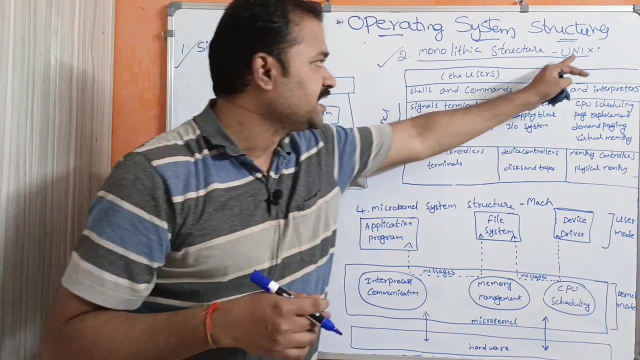 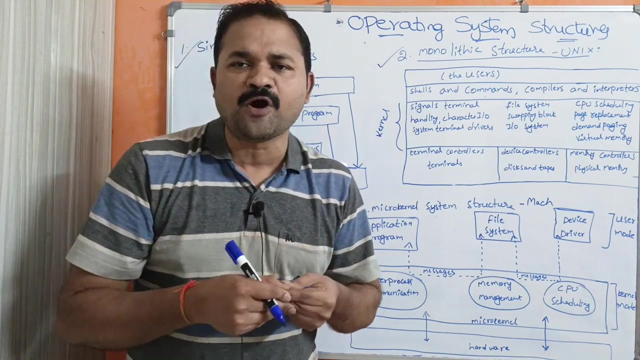 crashes, then there is a possibility that the entire system may fail. so this is the problem with simple structure. now let us see about the second one, that is, monolithic structure. the best example for the monolithic structure is unix. in this structure we have a kernel which performs all functionalities. 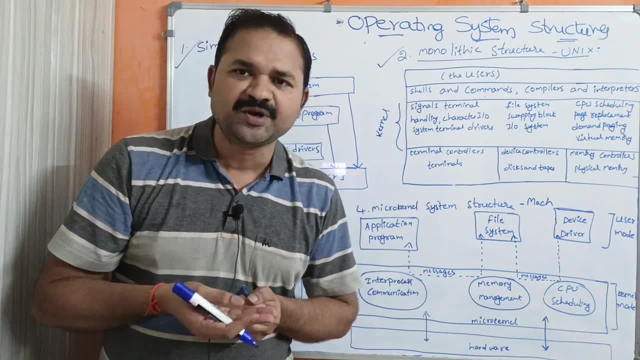 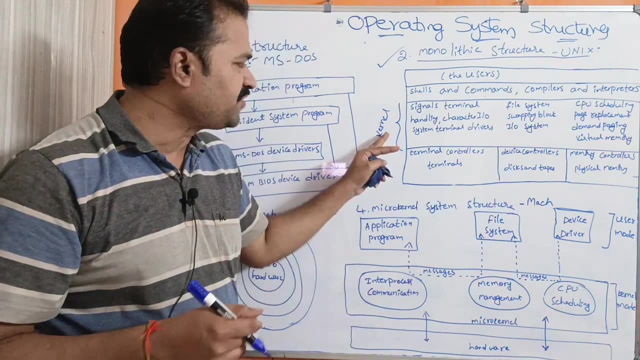 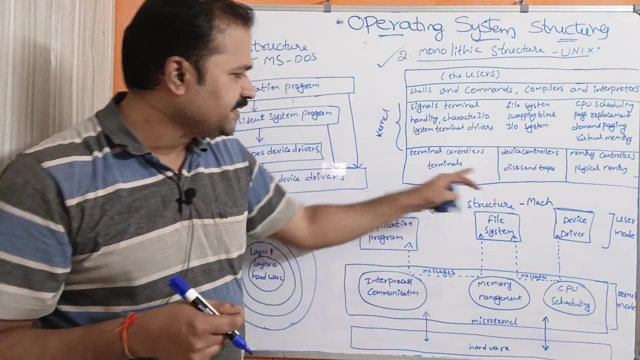 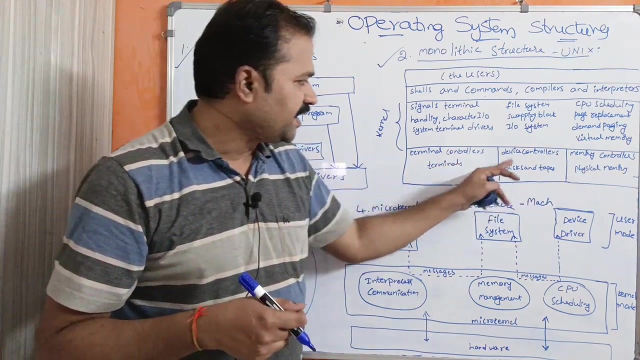 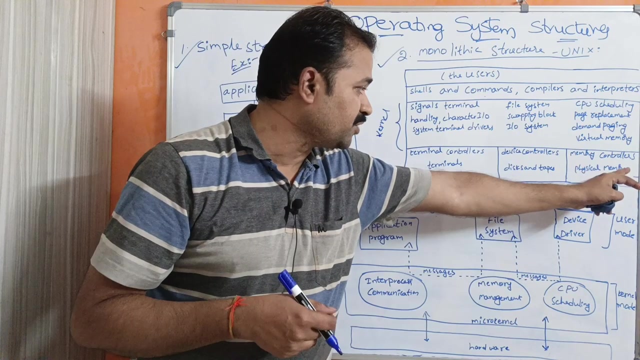 like process management, memory management, file management, i jer management, protection and security. so here we have kernel. kernel will do all the functionalities here, the monolithic here, if you observe, here at the bottom we have hardware devices. all these are nothing but hardware devices: Terminal controllers, next device controllers, disk and tapes, memory controllers, physical memory memory. 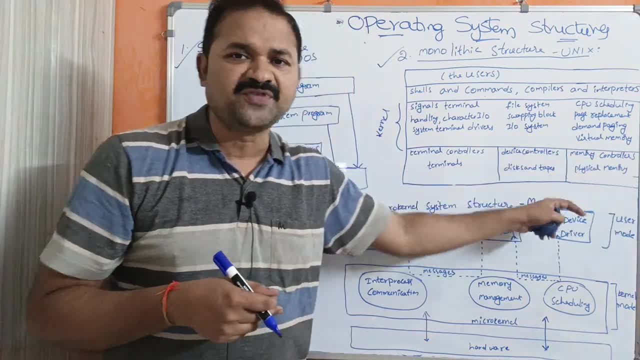 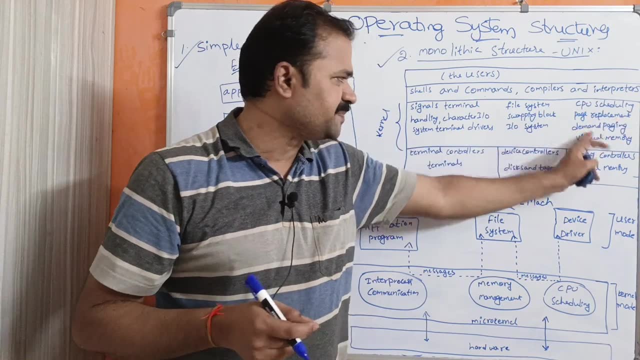 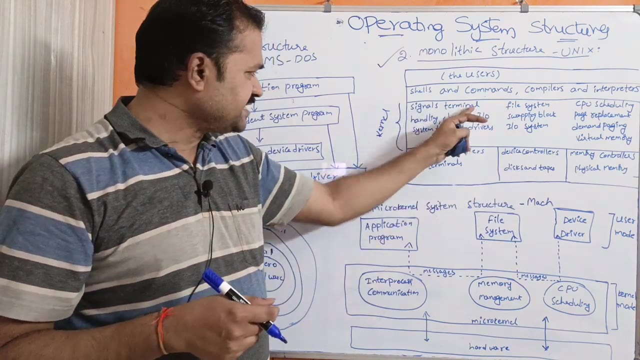 controllers. all this is nothing but hardware. on top of the hardware we have kernel. so kernel contains various functionalities like cpu scheduling page, replacement demand page, virtual memory file system, swapping block i o system, next signals, terminal, handling, character i o system, terminal drivers. on top of this we have 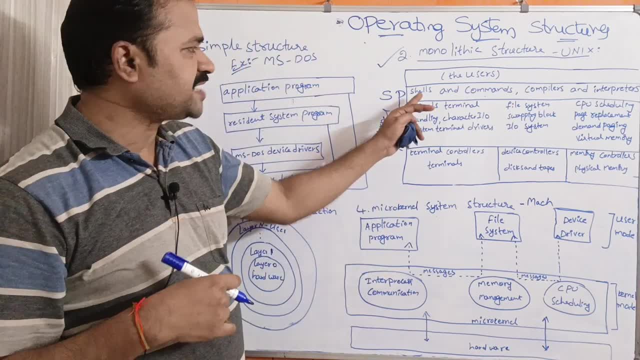 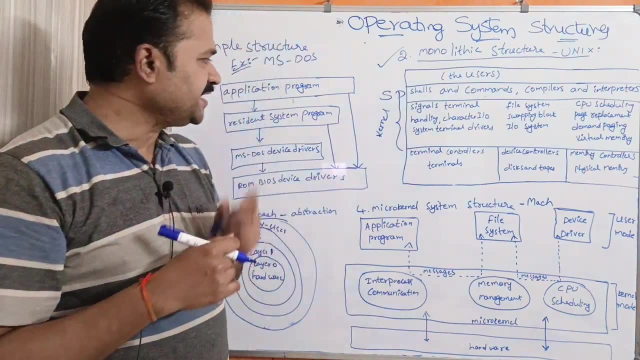 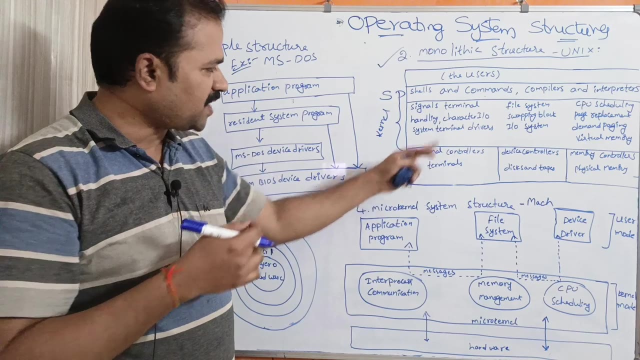 system programs. so we have system programs like shells, commands, compilers and interpreters. on top of it we have users. so here we can divide the monolithic structure into mainly two parts. we have some more parts also, but mainly two parts. the first one is kernel, the second one is system. 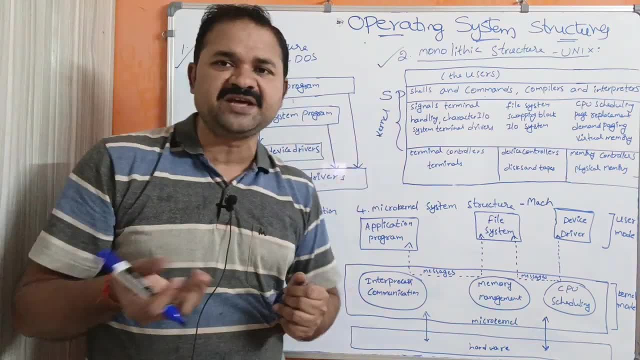 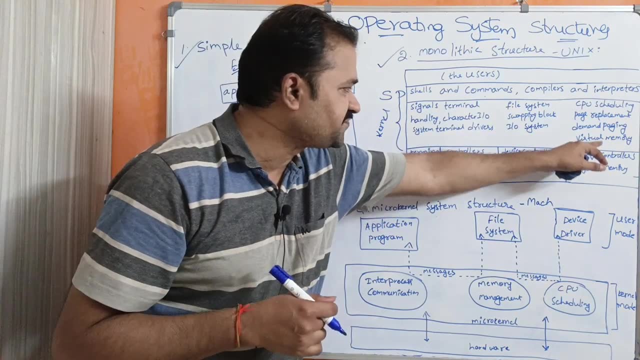 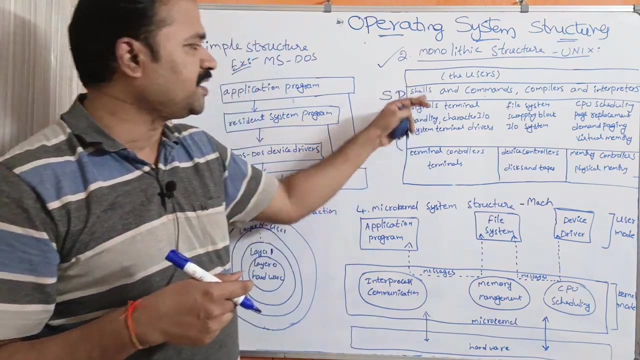 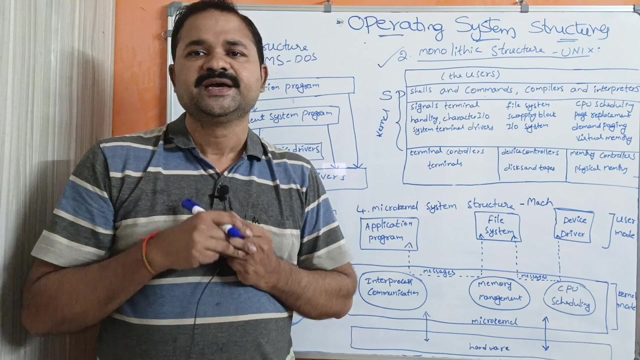 program kernel, again subdivided into two parts. the first one is device drivers. all these are nothing but device drivers. the second one is functionalities. all these are nothing but functionalities. functionalities, system programs. we have system programs called shells, compilers, interpreters and assemblers. here the major problem is if you want to add an extra functionality to the kernel. 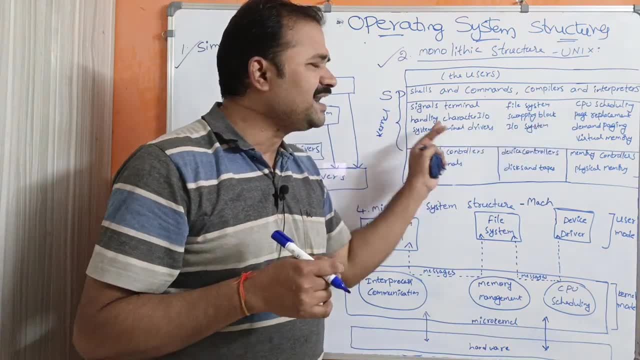 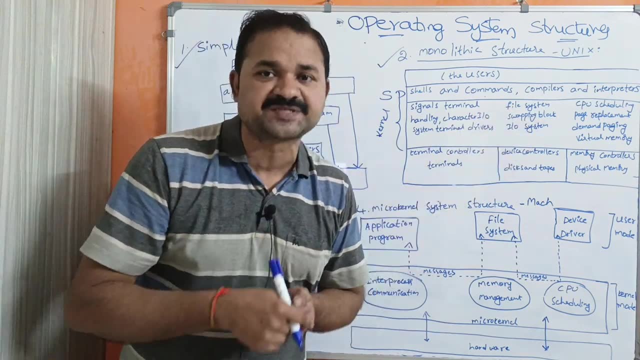 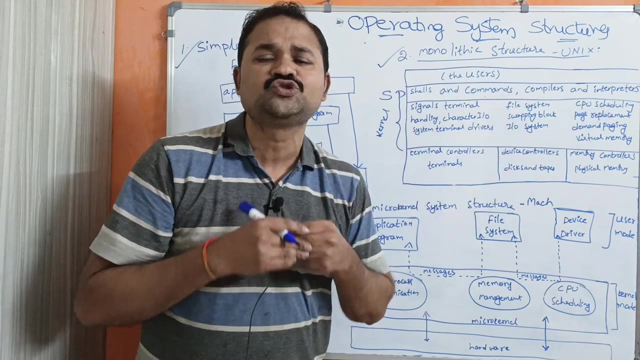 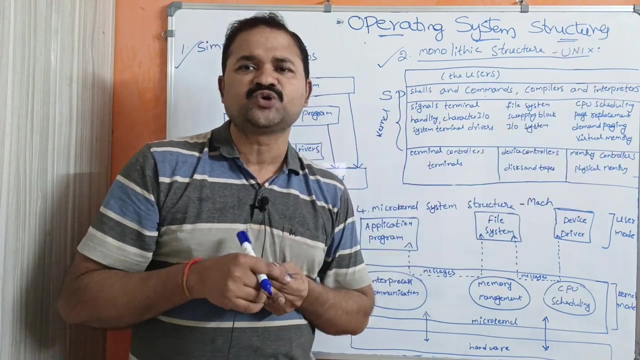 then what will happen is already kernel has too many components, so if you want to add a new component, then it will becomes. the kernel will becomes quite large and complex. why? because already the kernel has too many components. if you want to add one more component, then the kernel will becomes quite large and complex. so it is very, very difficult to implement. 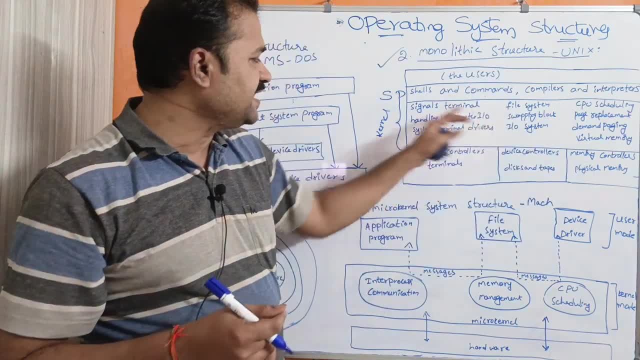 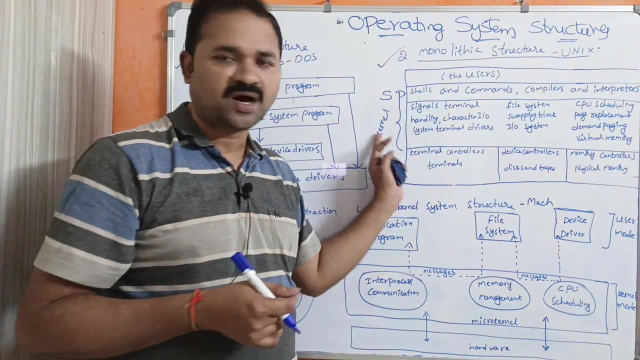 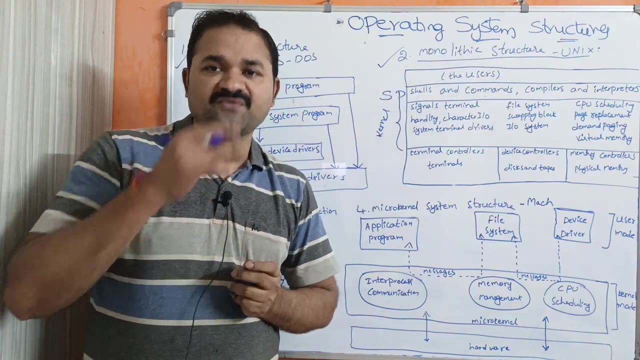 so this is the problem here. so here where the kernel resides, kernel resides on top of the hardware and on bottom of the system program. on top of the hardware and on bottom of the system program. what is the problem with monolithic structure if you want to add a new component to the system program? 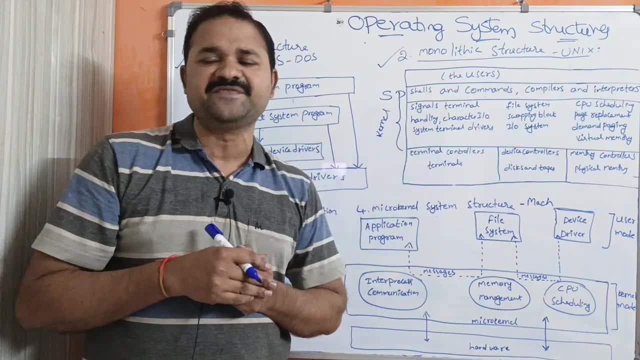 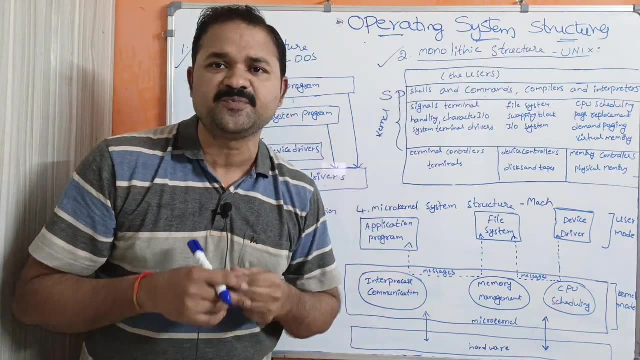 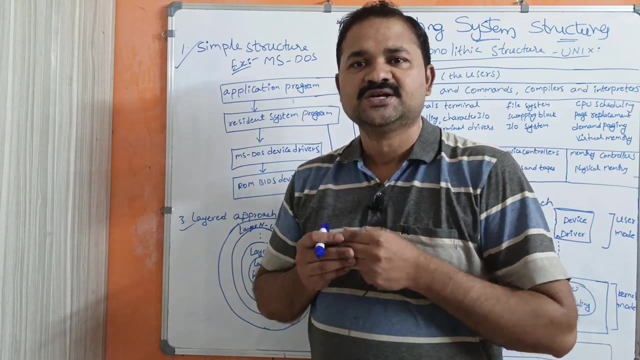 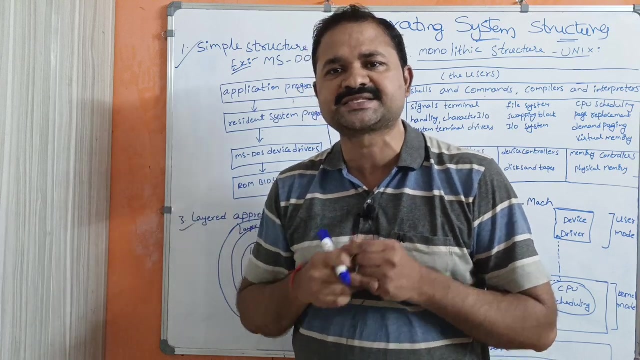 then when you add an extra functionality to the kernel, then it is extremely difficult. why? because already kernel has too many components. so this is about monolithic structure. the best example is unix operating system. now let us see the third one. the third one is layered structure. so in this structure, ah, we have several modules, so where each module is called as a layer. here we have several layers. the bottom layer is layered and at the bottom layer we have almost a whole layerrich consists of multiple layers, which is called layering. so here, the bottom layer, we have models. the modules are called layers. here we have several layers, the bottom layer is layered. is, and then we have comparative grouping modules, but you can even call it layers, say the bottom layer is различ senate structure. so this that we have mainly, we put two layers of it, which is이는 end. you can add a single layer here when the end customer anterior. you'll have views of the last Toni. 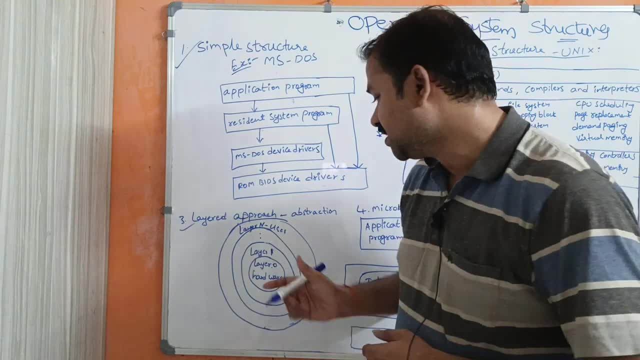 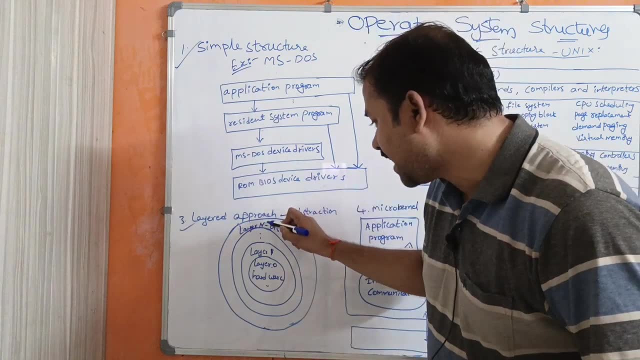 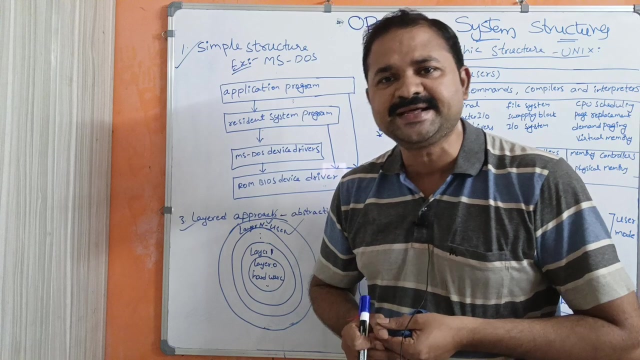 0. layer 0 represents hardware. on top of layer 0, we have layer 1 on top of layer 1, we have layer 2, likewise, and the highest layer, that is the top most layer, is layer n. layer n represents user. so here the point is, the bottom most layer is layer 0. layer 0 represents hardware, whereas the 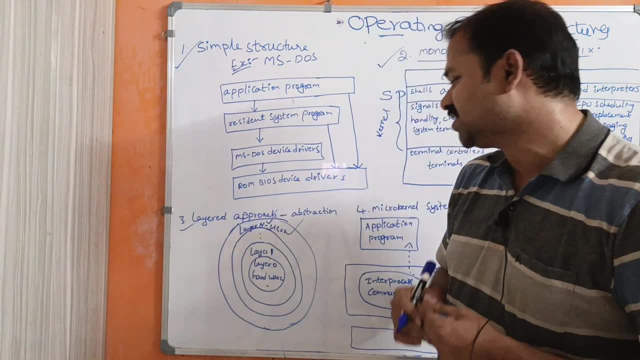 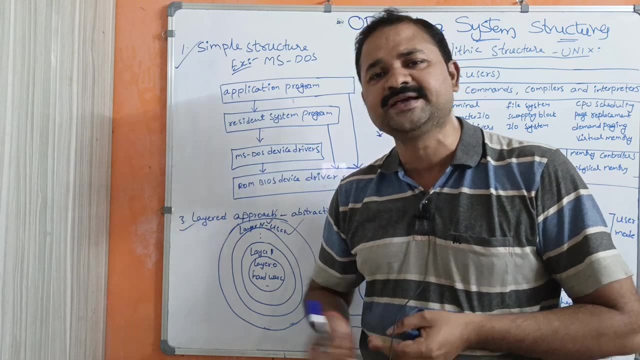 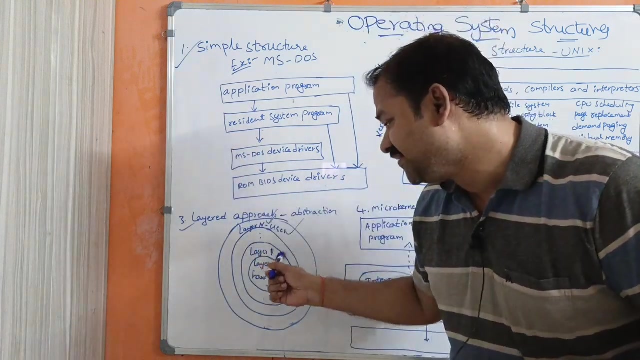 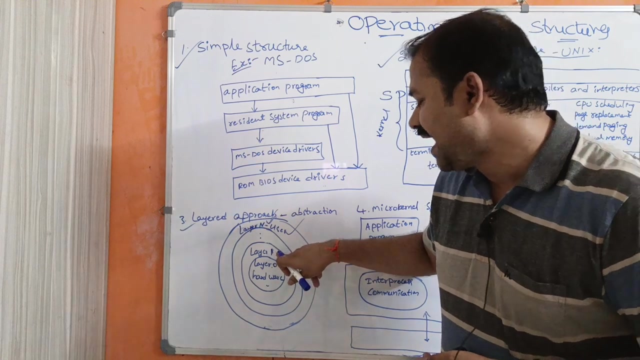 top most layer is layer n. layer n represents users. here each layer uses the services provided by its lower layers and provide those services to its upper layers. if you take layer one, layer 1 uses the services provided by layer 0 and layer 1 provides all those services to. 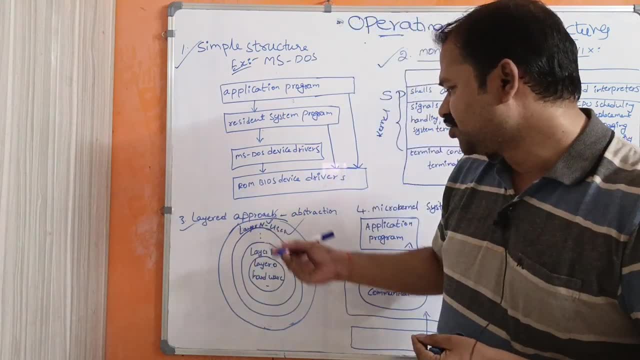 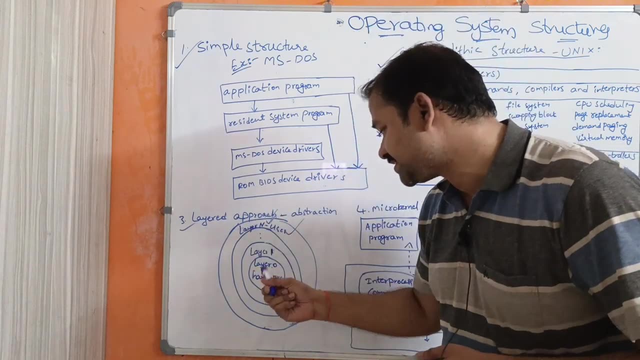 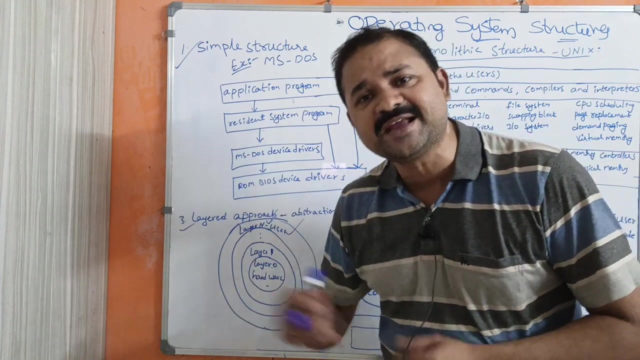 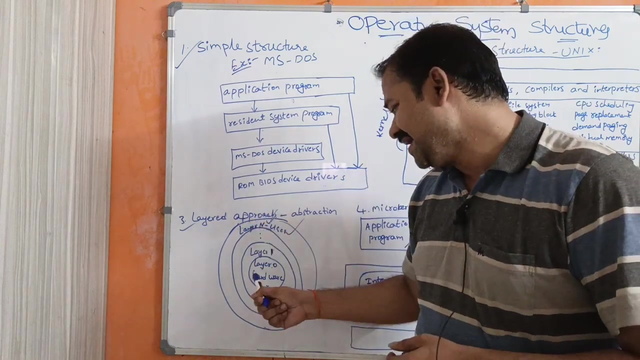 layer 2. so that is point here. so here the major advantage is: layer n, that is the topmost layer, cannot access layer 0, that is hardware, directly. why? because here layer n can access only layer n minus 1. layer n minus 1 can access only layer n minus 2, but layer n has no direct access with hardware. so that is. 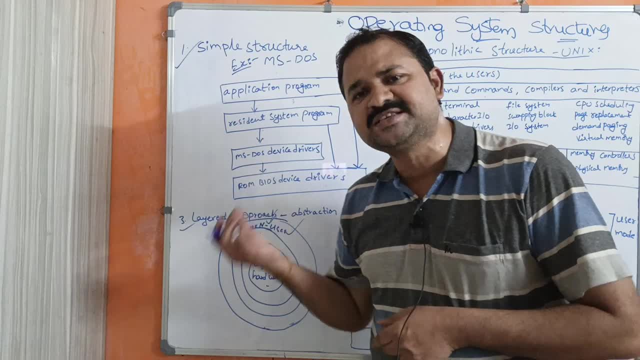 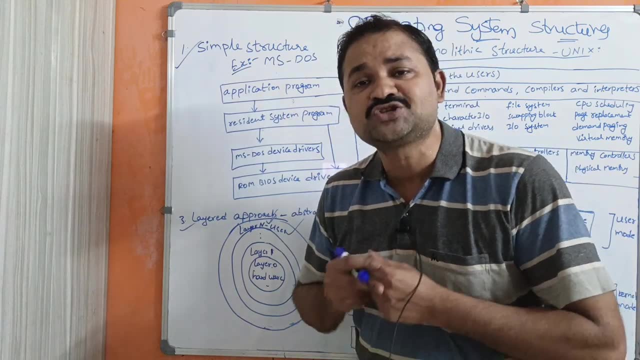 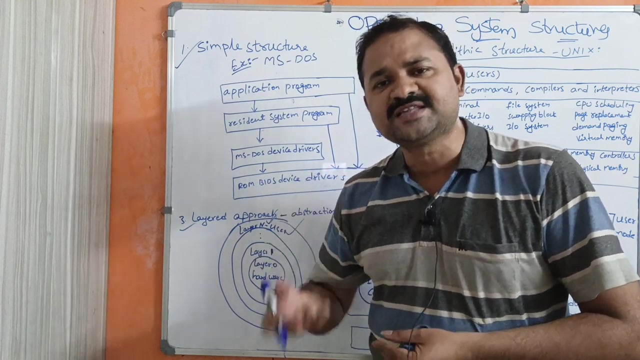 the advantage here? the main advantage of this approach is it is very, very simple to construct as well, as debugging is also very, very easy. what is debugging? debugging means it is the process of checking whether the program is producing correct output or not. suppose if there is a problem at 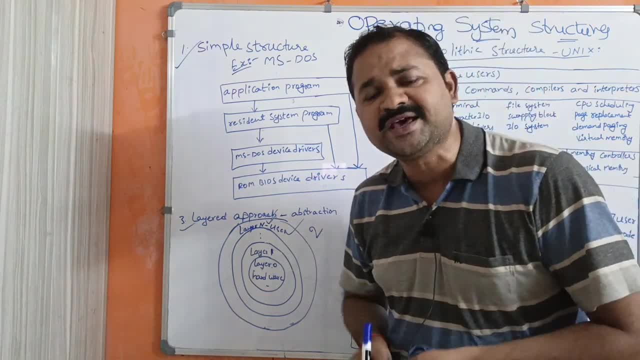 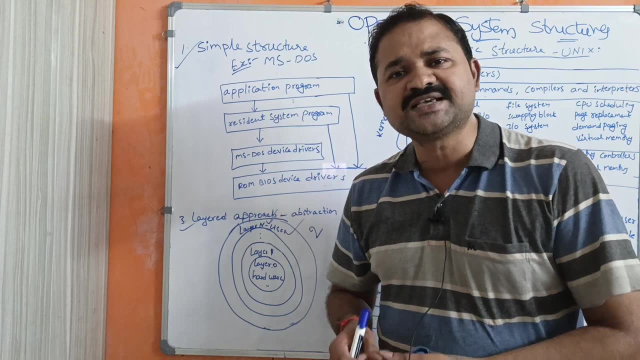 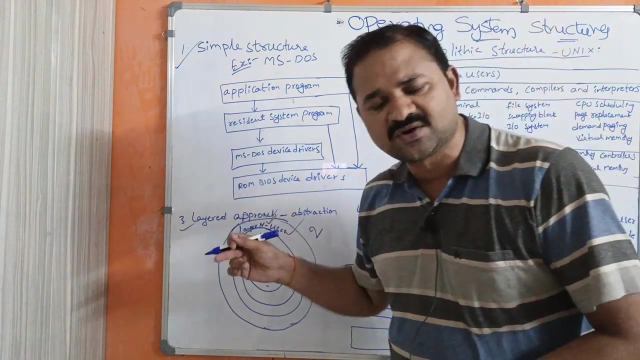 layer 2, suppose. if there is a problem yet layer 2, then we can say that there is no problem yet its lower layers, such as layer 1 and layer 0, and there are no problems yet its upper layers, such as layer 3, layer 4, likewise. so if layer 2 has a debugging problem, then we can say: 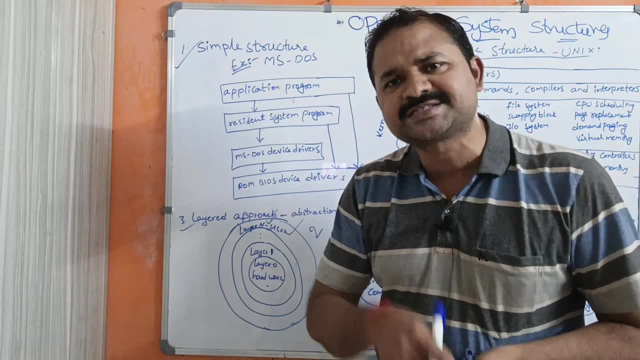 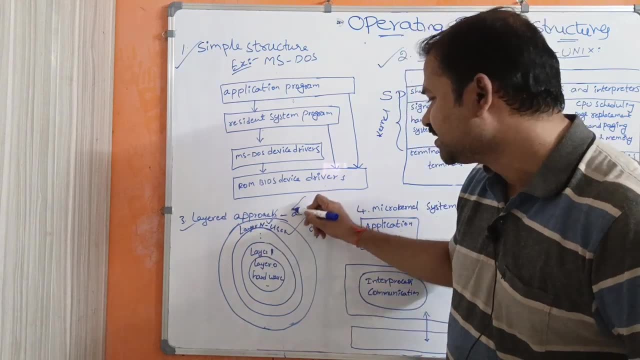 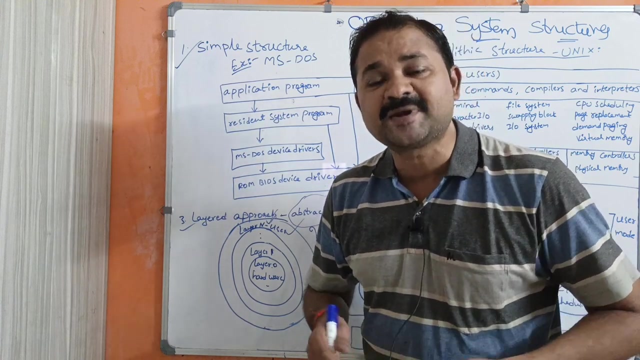 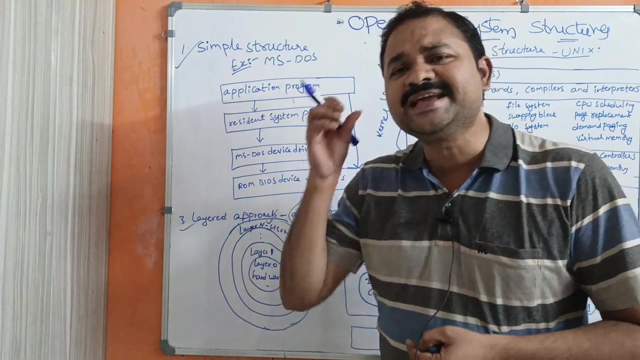 that only layer 2 has the problem. its lower layers and its upper layers have no problem. and the major advent? one more advantage of the layered approach is it implements abstraction. we know what is abstraction. abstraction means showing, representing essential features, and hiding the background details, unwanted details. here each layer uses the services. 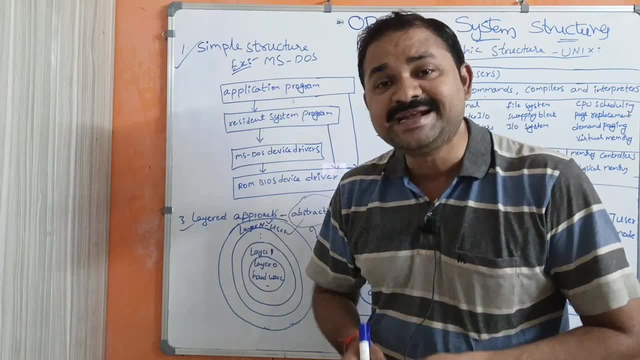 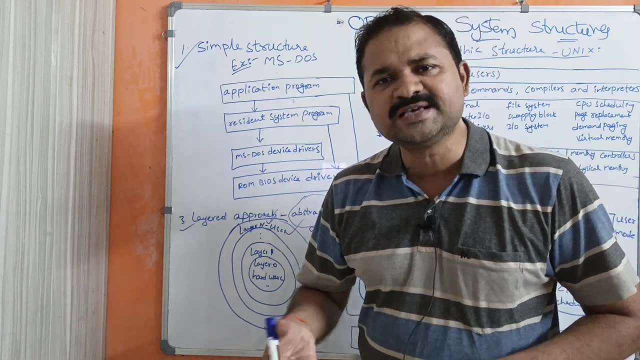 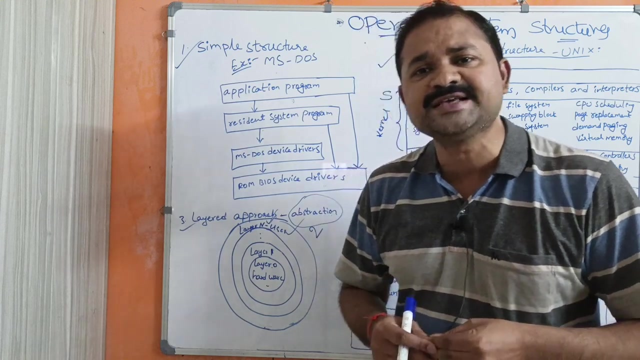 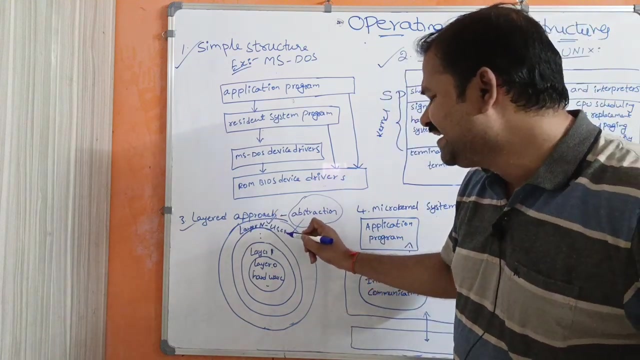 provided by its lower layers, but it doesn't know how all those services are implemented. so layer 1 can uses the services of layer 0, but layer 1 doesn't know how layer 0 is internally implemented. and the major disadvantage of this approach is it is very, very difficult to design all these layers. why? because here we have too many layers. 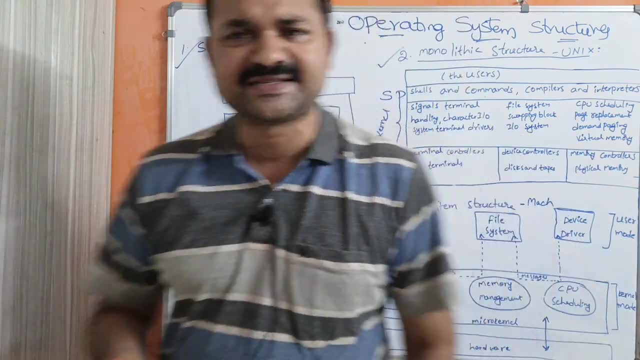 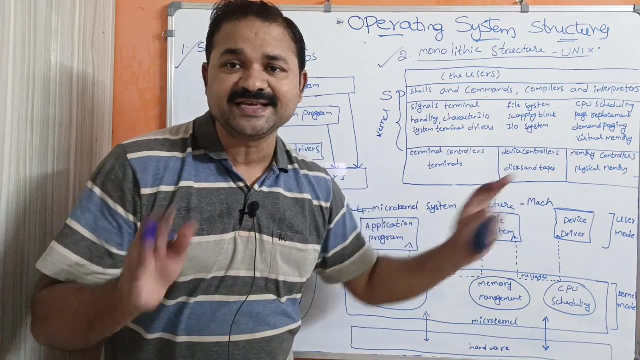 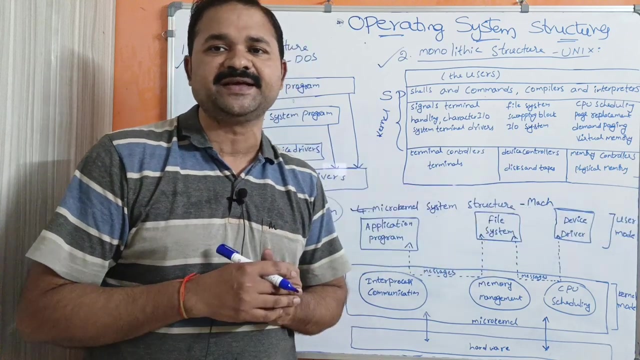 so designing of those layers are difficult. so that is the disadvantage here. and the fourth one is micro kernel structure. the best example is mac. it is not apple mac, it is mach. in the olden days we use mseh operating system, whereas the apple mac spelling is mse. here micro. 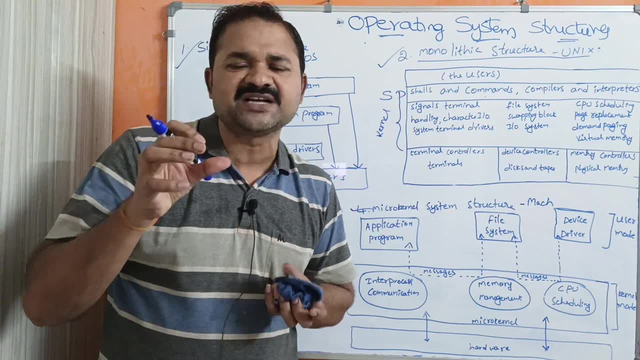 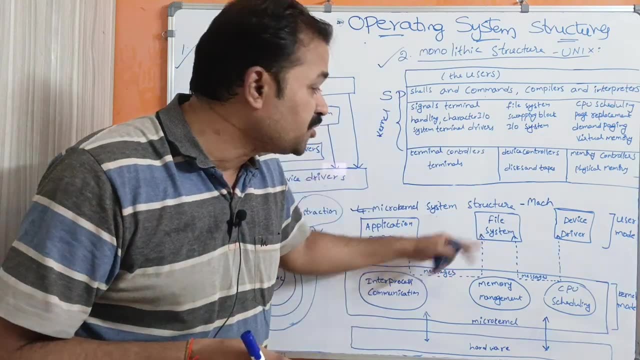 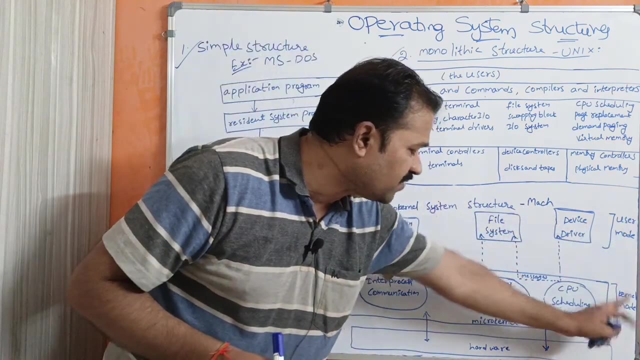 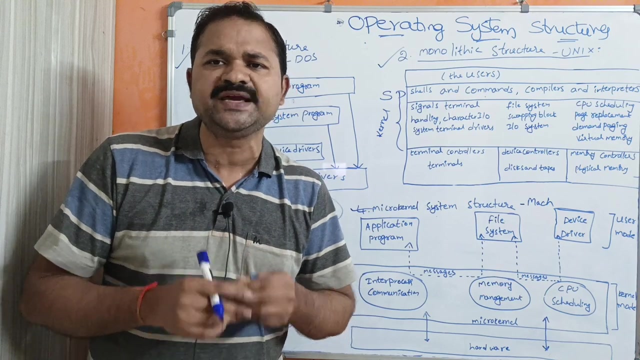 kernel means uh. the important functionalities will be placed in the kernel and the unnecessary details will be pushed on to the user mode. here we have user mode. user mode means user programs. here we have kernel mode. so kernel node mode means micro kernel, uh. here micro kernel contains only the necessary components, important components such as ipc memory. 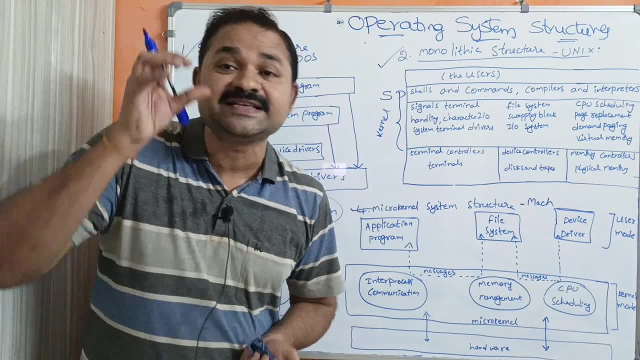 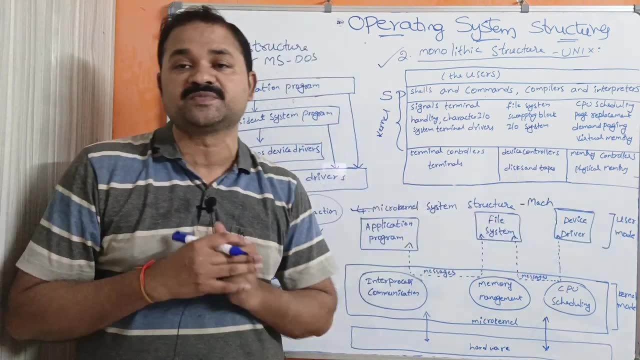 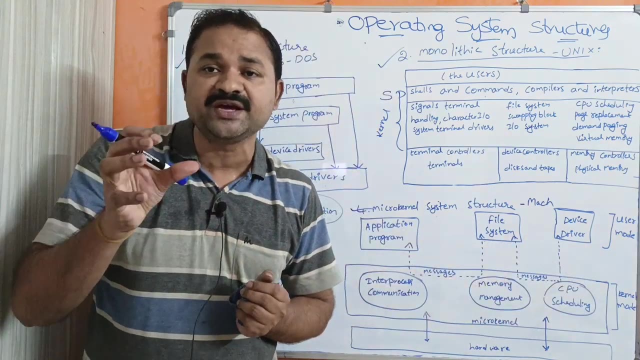 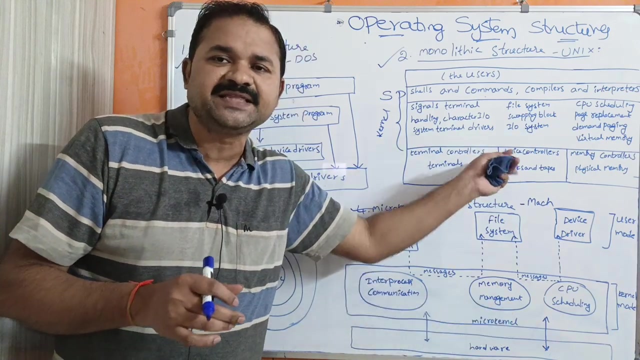 management, cpu scheduling. various unnecessary components of micro kernel are moved to the user user programs. so the code will become small in the micro kernel. why? because here what we are doing, we are removing unnecessary functionalities of the kernel and we are placing them in user programs. so the the size of the 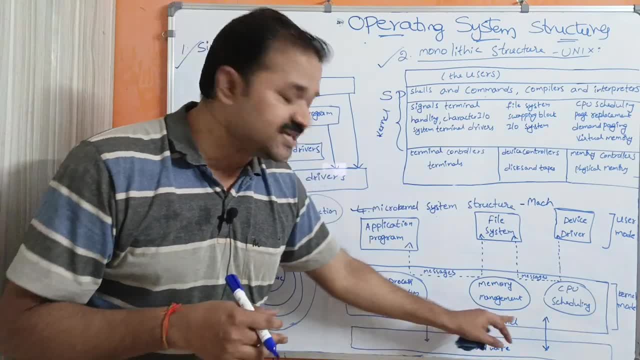 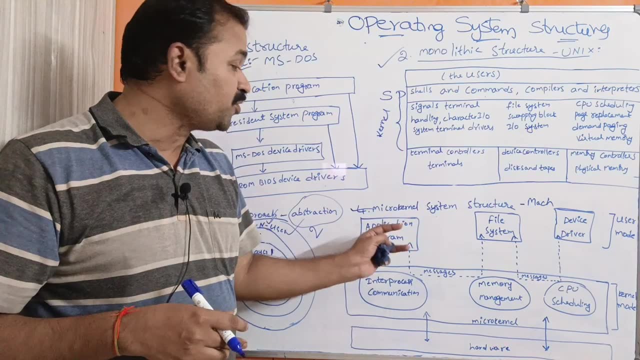 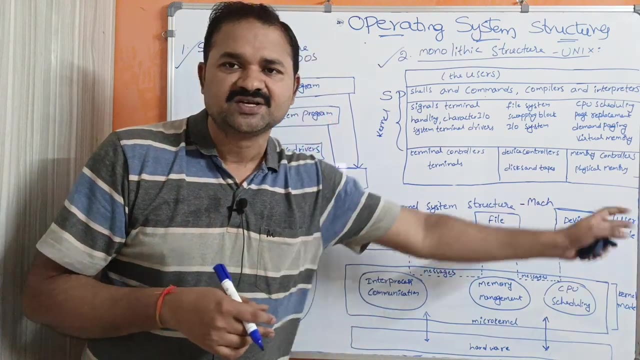 kernel will becomes quite easy. so that's why it is called as micro. so micro means small. it contains only necessary components. so the remaining components are available in user programs, like we have: application program, file system and device drivers. so all these are nothing but unnecessary components of the uh. this. 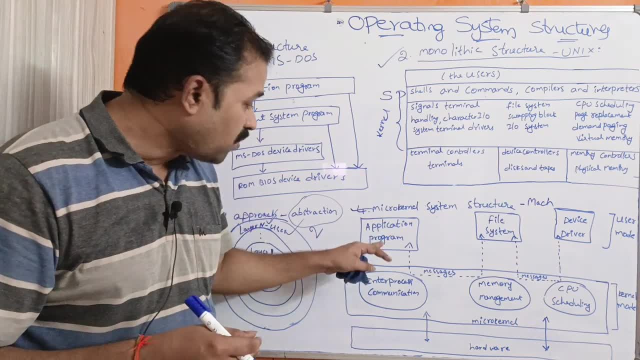 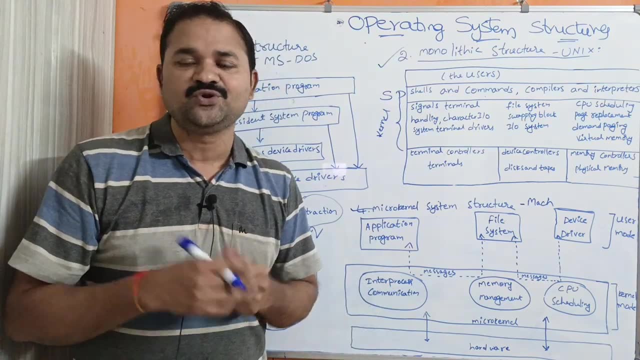 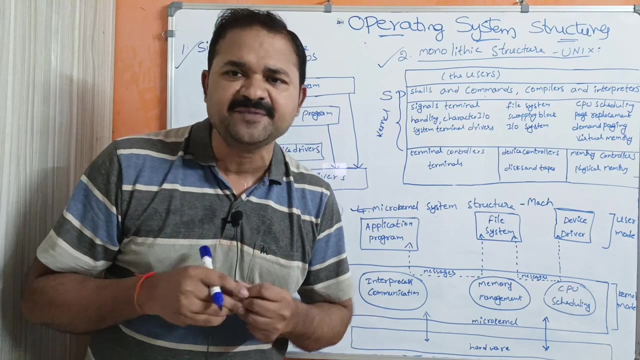 okay, this is nothing but micro kernel. so here one user program can interact with another user program with the help of ipc. we know about ipc inter process communication. one process can communicate with another process with the help of the ipc. so here application program can interact with file. 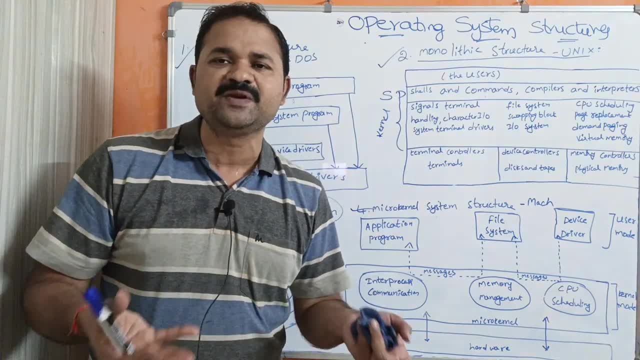 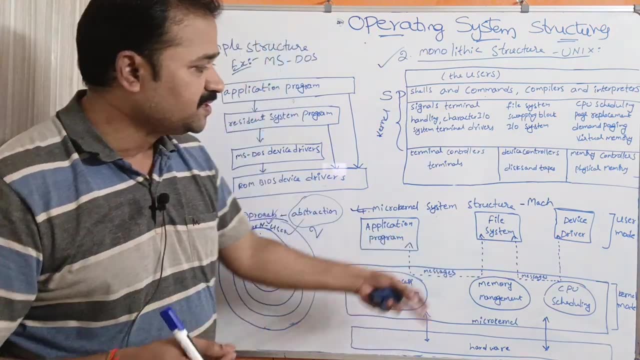 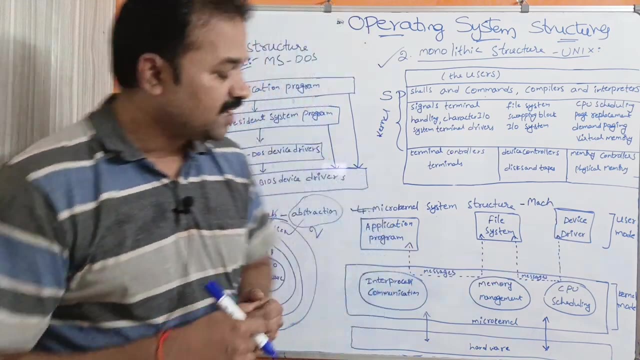 system with the help of ipc. we know that we can implement ipc with the help of message passing, so application program is sending messages to the file system. likewise, file system can interact with device device drivers with the with the help of some messages. okay, and the problem with this approach is here. here the user programs.